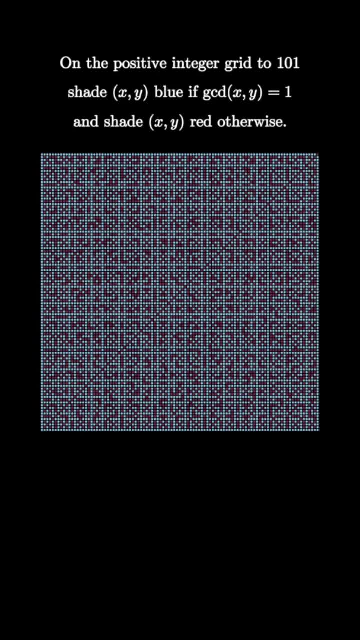 that the quantity 6 over pi squared is approximately equal to the ratio of the number of blue dots to total dots. It turns out in this picture: there are 6287 blue dots and 10201 total dots. This means that 6 over pi squared is approximately 0.61631,. 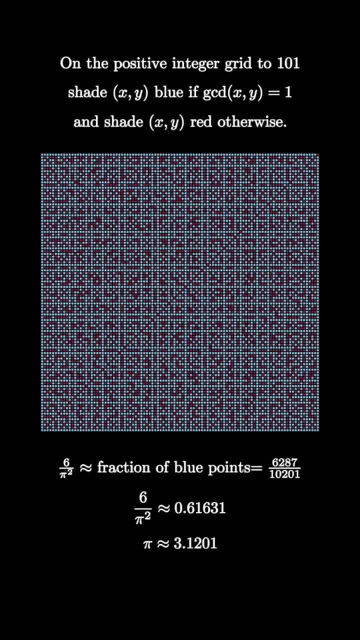 and from this we conclude that pi is approximately 3.12.. Not the best approximation, but definitely a fun and beautiful one. 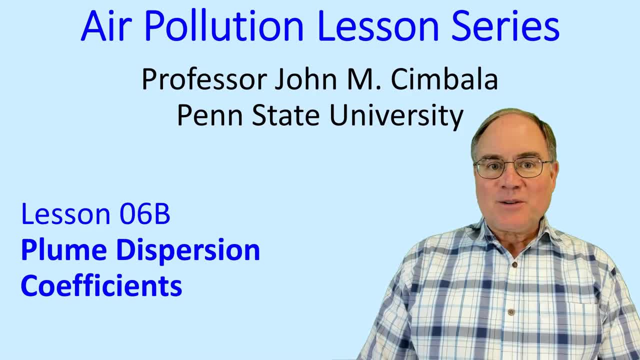 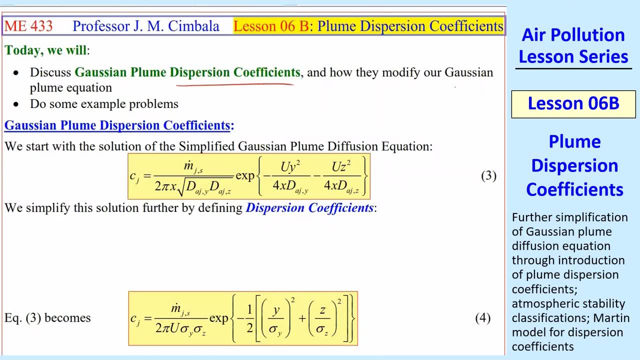 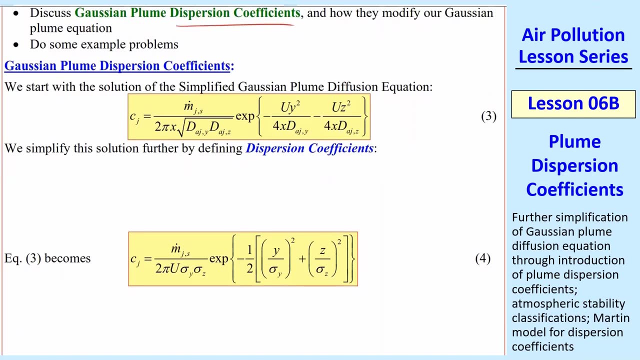 Welcome to Lesson 6b: Plume Dispersion Coefficients. We're going to introduce something called dispersion coefficients that will be able to modify our Gaussian plume equation and then we'll do some example problems. Here's the equation we had from last lesson- I called it the simplified Gaussian plume diffusion equation- which was equation 3 in our numbering system. 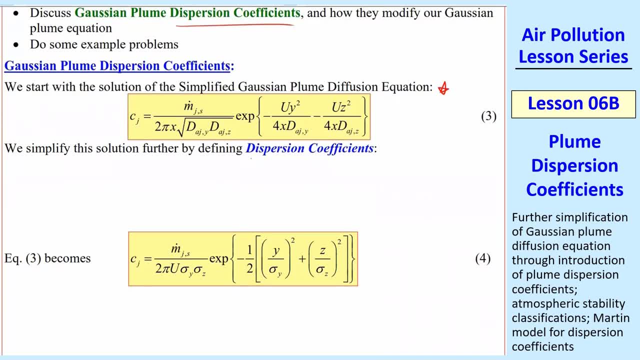 We can simplify that further by defining something called dispersion coefficients. We're going to define two of them. Sigma y is defined as square root of the quantity, 2 times x, times d aj y over u. and then sigma z is defined in the same way, except with d? aj z. 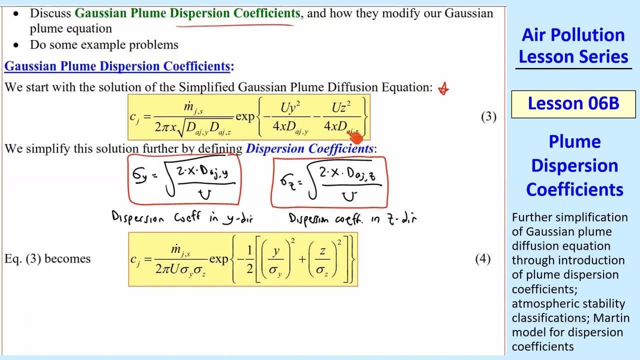 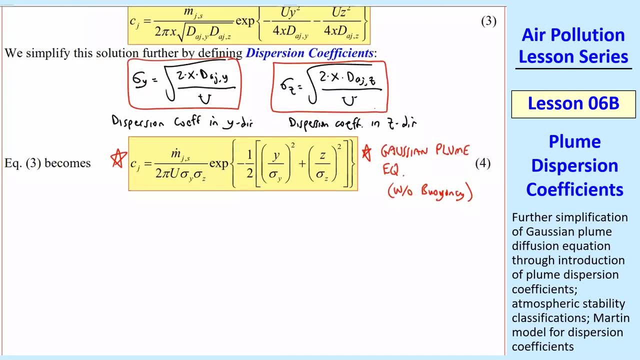 What we're doing basically is combining some of these terms. here There's an x, d, aj, z and a? u. In other words, when you plug these into here, you can reduce equation 3 to the Gaussian plume equation, but it does not have to be the same. 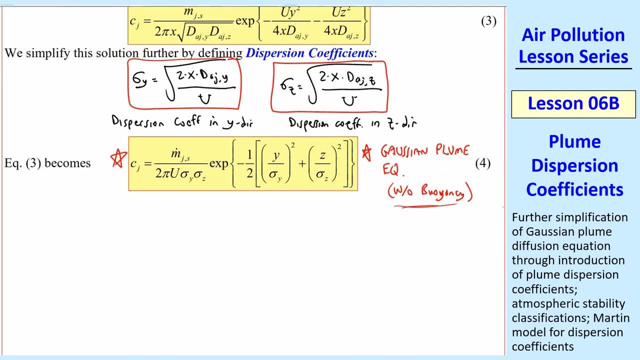 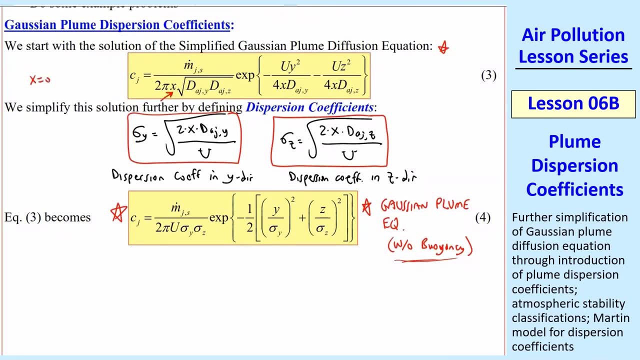 We don't have to have buoyancy. We're still not accounting for buoyancy. And I just wanted to point out one thing here: In our original equation- remember- we had this x in the denominator. So x equals 0, is a singularity, Cj goes to infinity. there We have a point source, so that makes sense. 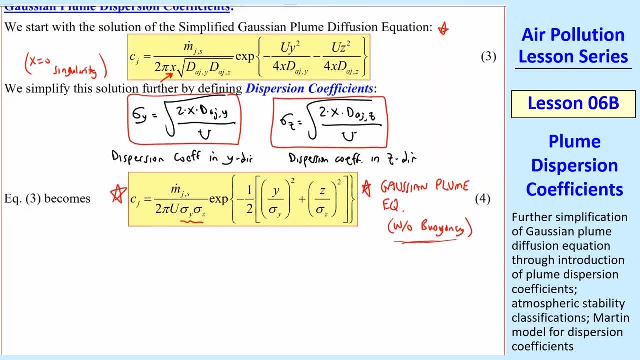 Well, we still have retained that because the sigma y and sigma z are in the denominator now, And sigma y has an x in the numerator. Sigma z has an x in the numerator- square root of x actually. So you still have your x in the denominator.